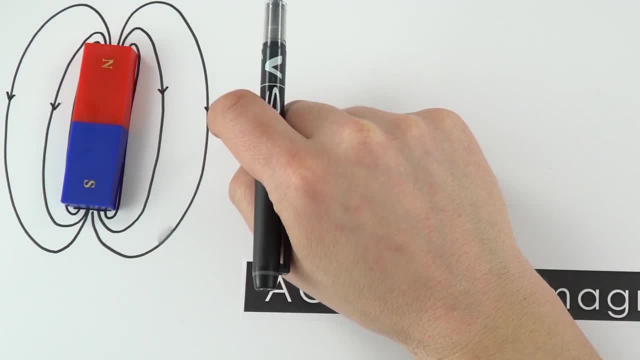 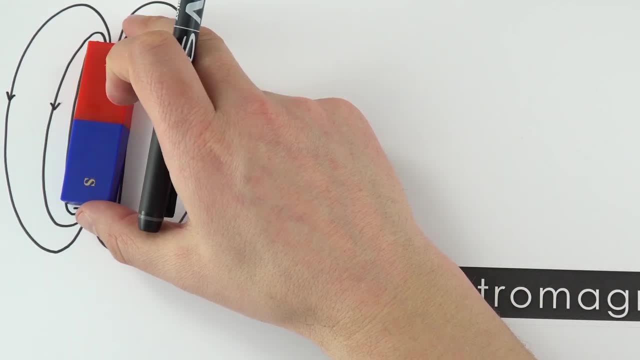 bar magnet. Now, this is also the shape of the magnetic field around the Earth And this is the reason why, if you have a compass, if you're navigating, it always points to north. So the evidence that we have this magnetic iron core in the center of the Earth is because 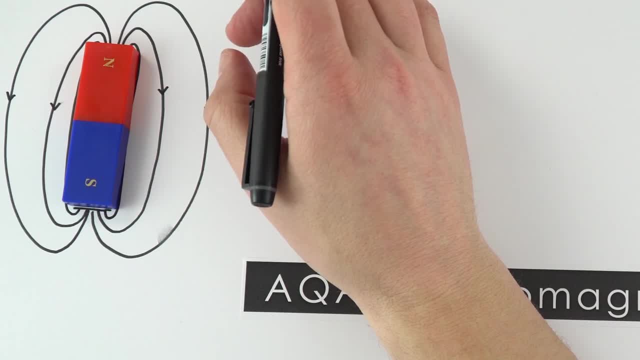 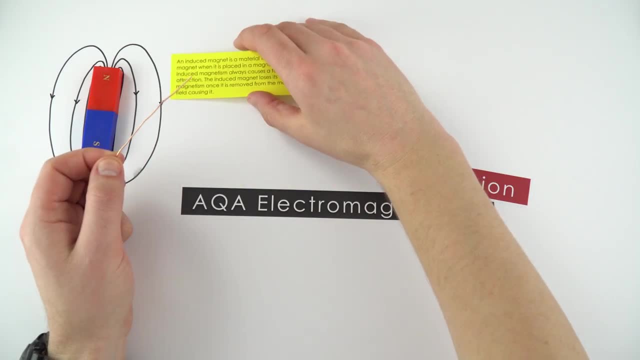 of the magnetic field that we can experience and actually detect every day. But something really happens if you have a piece of wire and you connect it into a circuit so that there's a current flowing. What we then have is what we call an induced magnet. So just by having a current flowing, 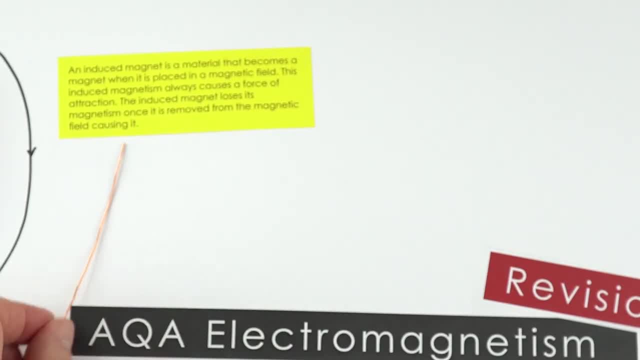 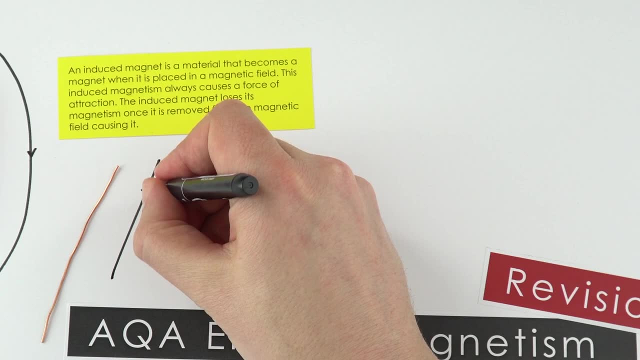 in a conductor. we then have a magnetic field. Now, if we have a conductor like this, which is just a wire, then if we actually start to look at the field lines, maybe you've got the current flowing in this direction. I'm just going to draw the field lines in green. 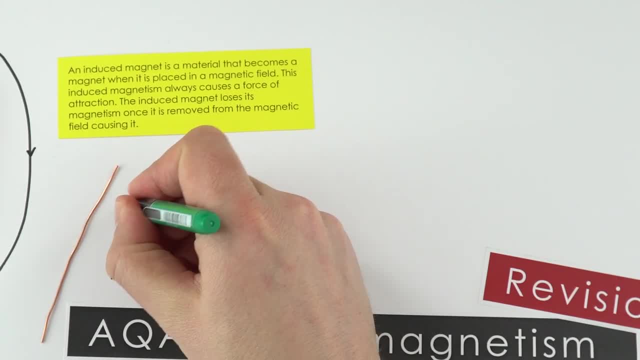 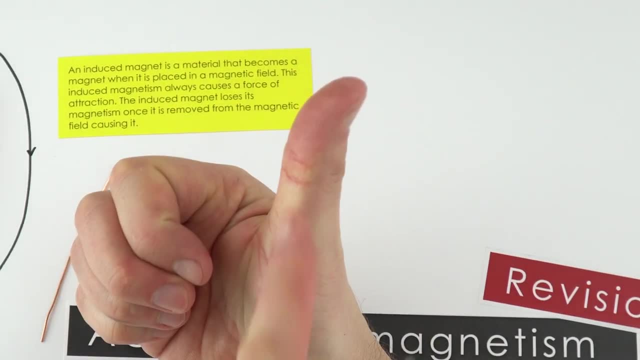 What we have are these concentric circles that get more and more widely spaced as we actually draw that, And we can actually think about the direction of this by using our right hand rule. So if this is the direction of the current, with my thumb, then my fingers. 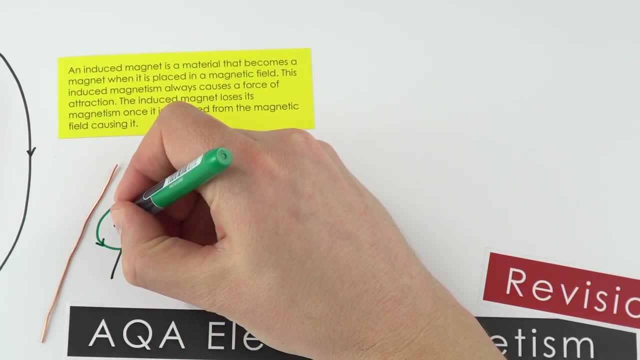 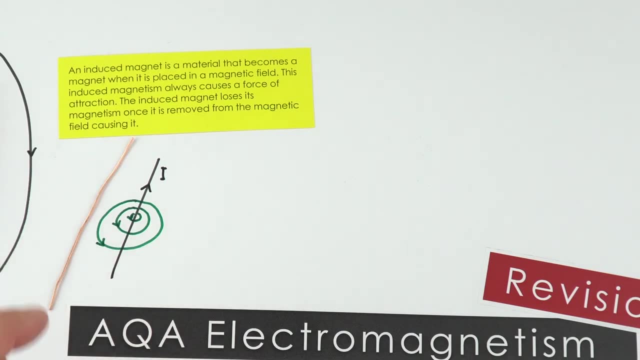 point in the direction that that field is going. So we have the field lines like this: I've just got an hour to show the direction of that field. Now the thing is, if we had more wires, then we'd have a stronger magnetic field And actually, 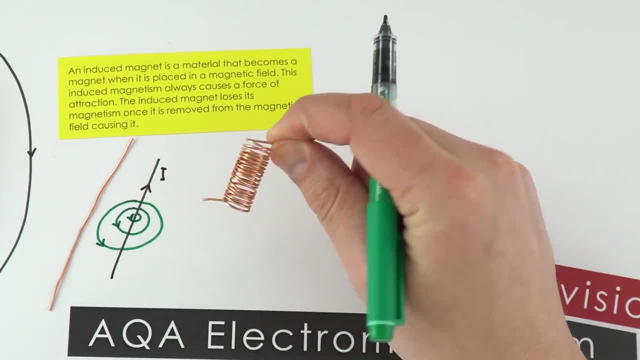 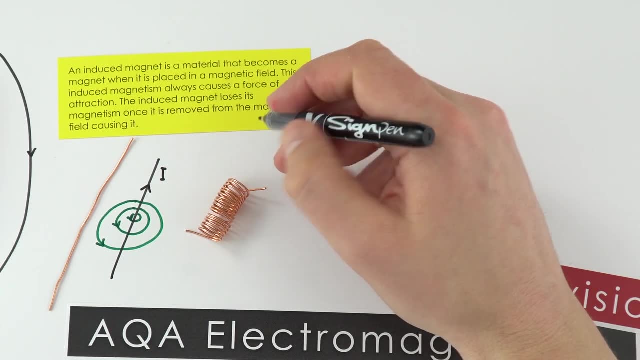 if we had it coiled round into a coil like this, we'd have an even stronger magnetic field. Now, this coil of wire here, which is a coil of wire that can carry a current, is called a solenoid, And if I was to draw a solenoid a bit like 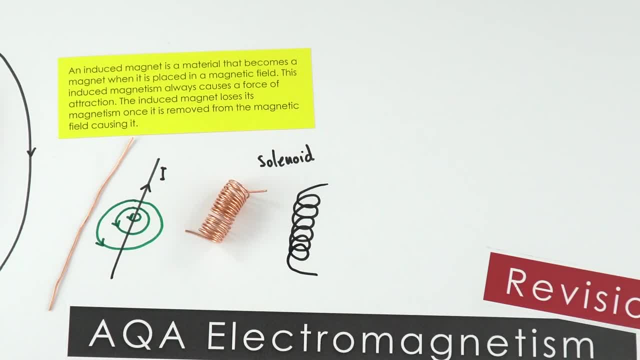 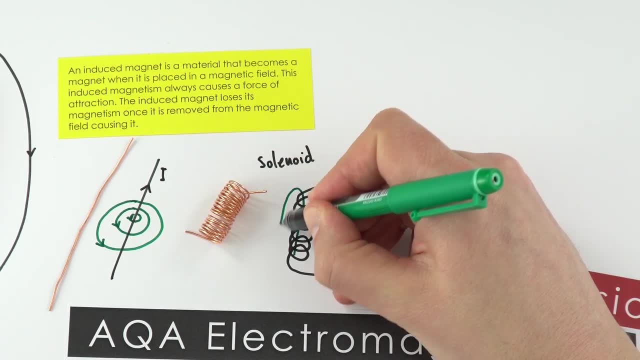 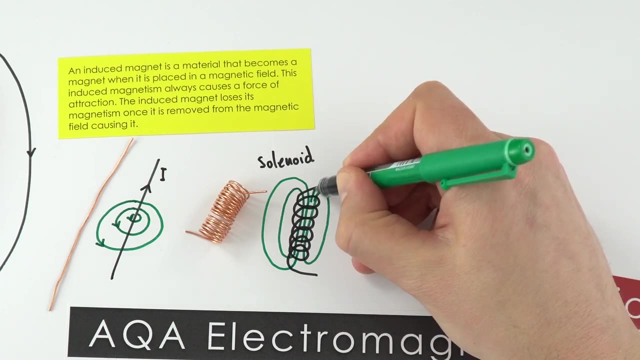 this. I could then draw the magnetic field lines through it And actually what we find is in the middle we have these lines which are really close together, like this, And they also come around the side, like that. In actual fact, this is the same shape as we have around. 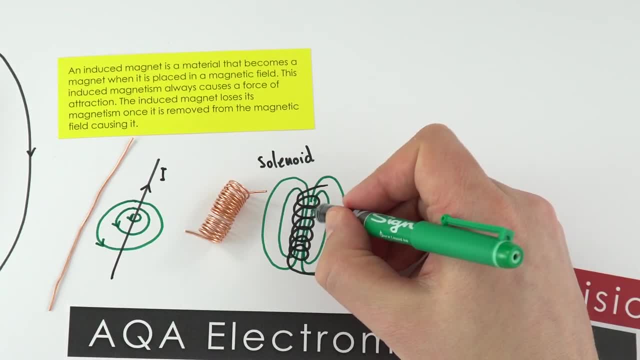 a permanent magnet over here, But in the middle we have this dense magnetic field where all the field lines are really close together. Again, these can go from north to south, And so in a solenoid what this behaves is when you put a current through it this behaves a bit like a bar magnet, And that's incredibly. 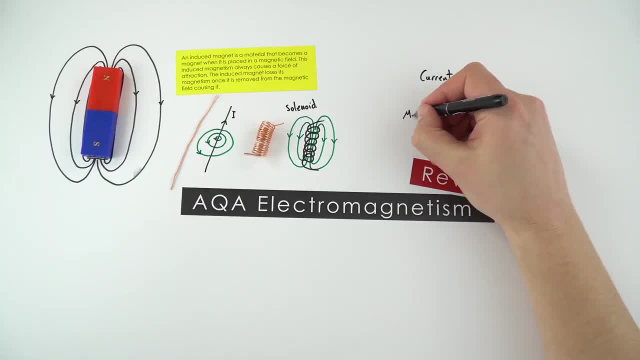 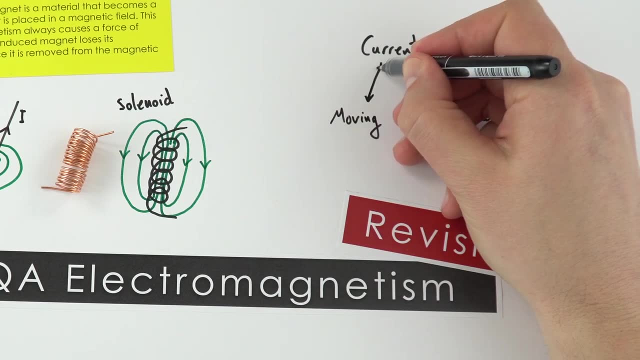 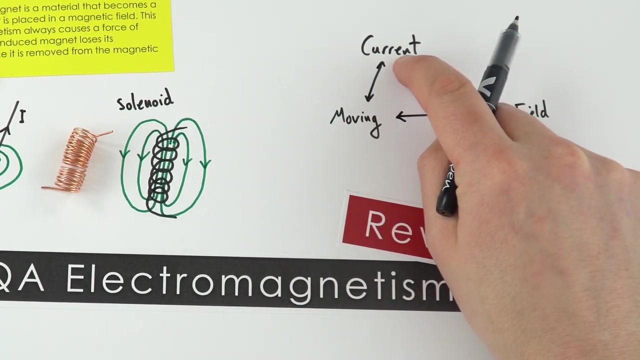 useful for all sorts of devices. Now, when you have a current and it's moving, this then causes there to be a magnetic field, And these three things are really closely linked to one another. So you have a current flowing, so there's a movement of electrons inside a wire. we 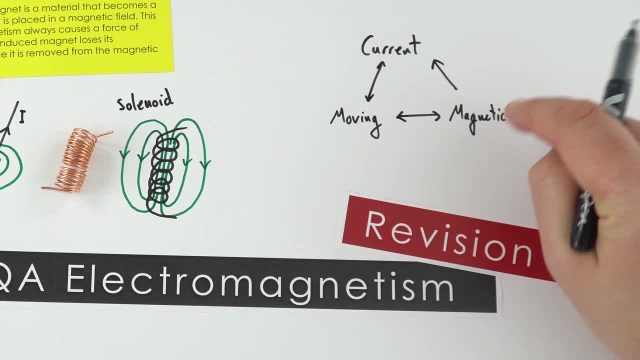 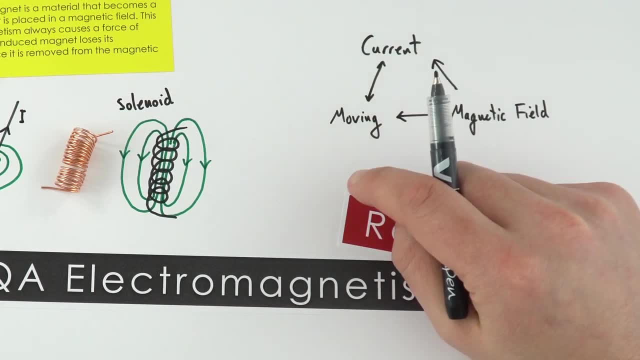 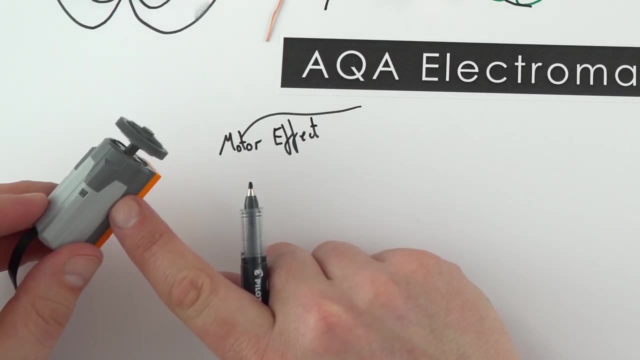 cause a magnetic field. But what would happen if we had a magnetic field and a current flowed in that? What you then get is the third side of the triangle. you get the movement, And this is called the motor effect. So the motor effect is put to good use in motors. What we have inside this motor here? 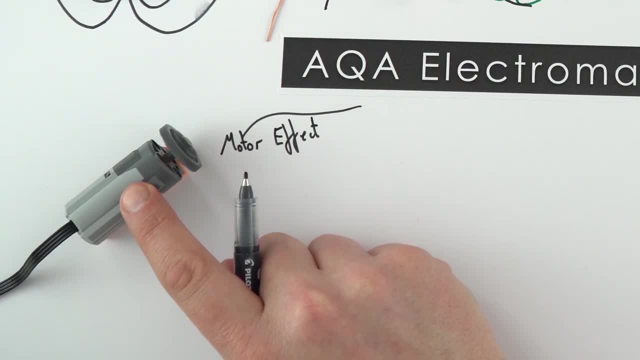 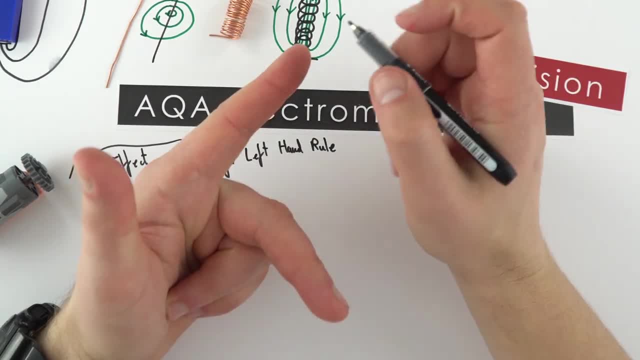 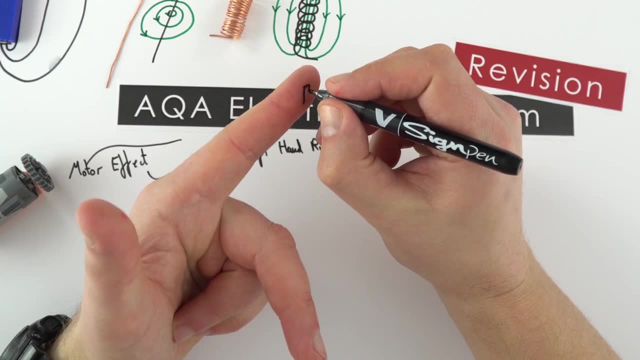 So we can actually use something called flow. So we have something called Fleming's Left-Hand Rule. Now for this. my first finger tells me the direction of the magnetic field- Now a magnetic field we actually give the symbol b to. My second finger tells me the direction of conventional current. 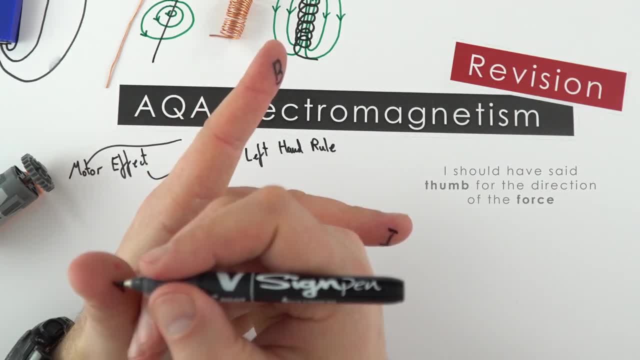 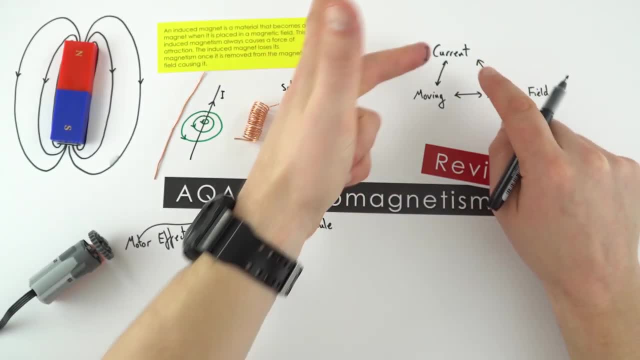 And my first finger tells me the direction of the force that a conductor's going to experience and therefore the direction it moves. So we can see that we've got from this triangle over here. we've got magnetic field, we've got current, and then my thumb is the force, or 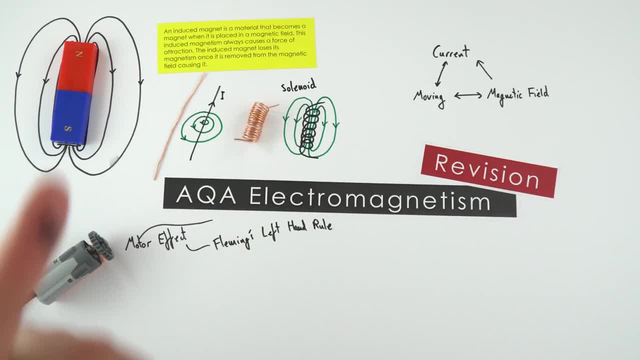 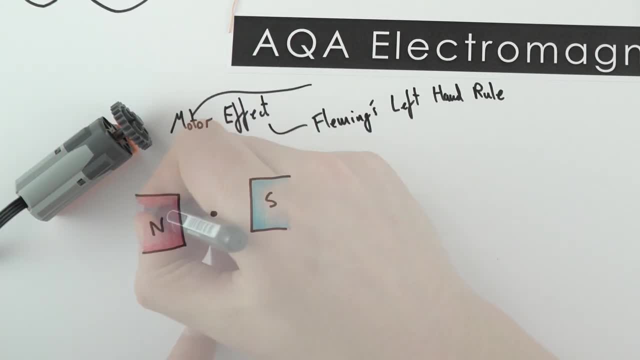 direction of that movement. So these three things are really closely linked. Now, what this means is that if you had just a single wire in a magnetic field, we could predict which way it's moving. So let's imagine we had the north end and the south end of a magnet. 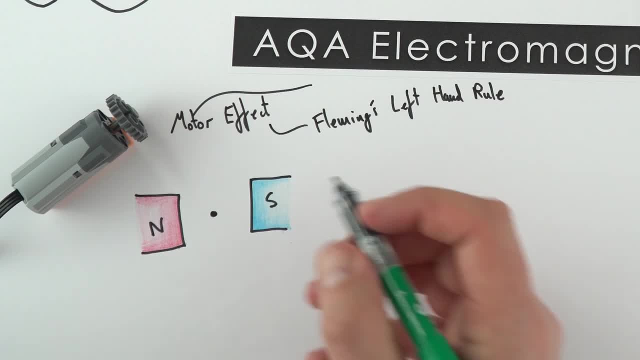 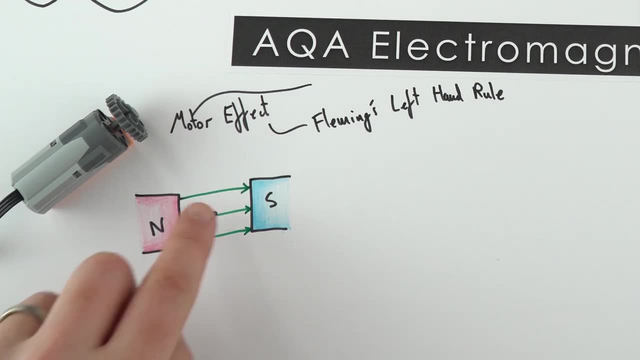 like this: Between the two of them, there's going to be a region where you have a magnetic field. I'm going to draw this in because we know that the magnetic field goes from north to south. Now this wire here is effectively coming out of the paper towards you. I've 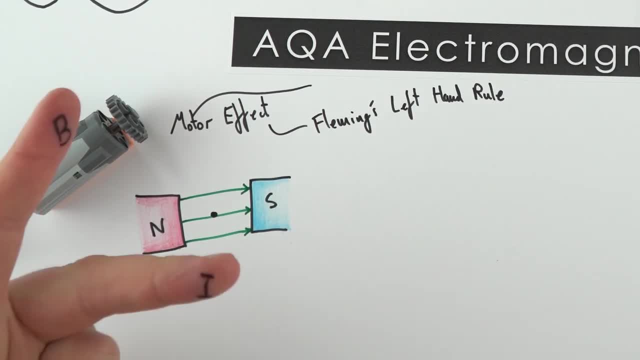 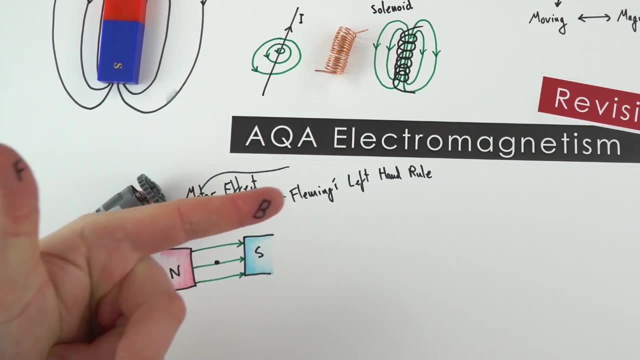 just drawn that with a dot. We can then use Fleming's left hand rule to predict which way that wire would move. So first of all, my first finger is a magnetic field going from north to south like this. My second finger is a current which is coming out of the paper. 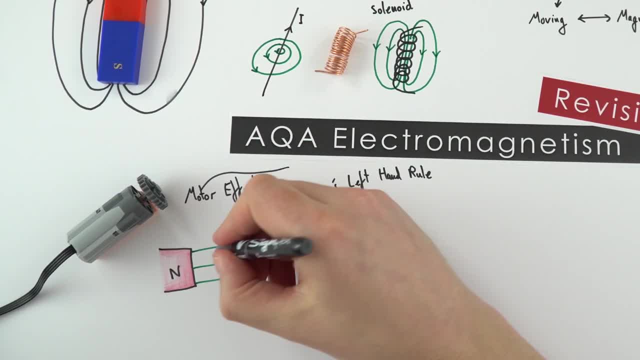 It's pretty awkward to do this, And my thumb is pointing up. So what we'd have here is the wire would move in this direction. Obviously, we could turn that wire to go downwards by either reversing the direction of the magnets or we could reverse the direction of that. 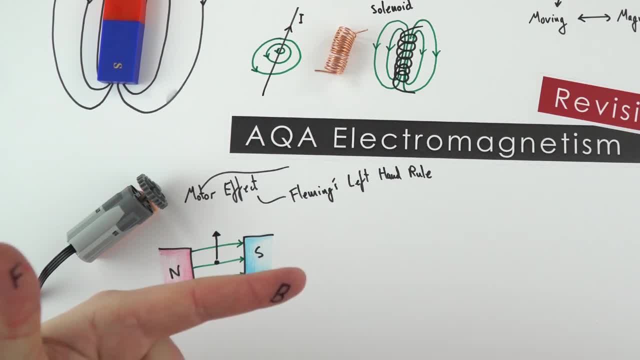 wire So we could either reverse the direction of that wire or reverse the direction of that current So effectively. what we're doing there is, if we were to reverse the direction of the magnet's magnetic field, this would happen and my thumb would point down. Really awkward to do If you're in an exam and you see people starting to. 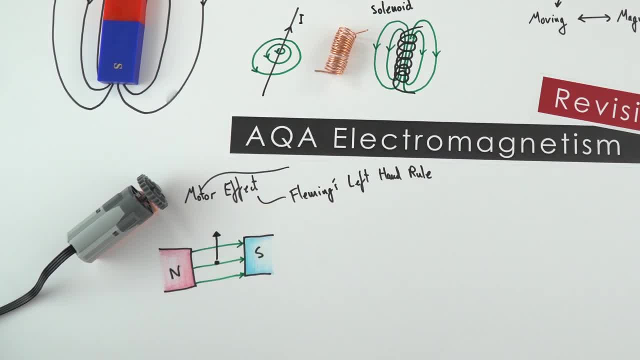 do this. there's probably a question about the motor effect and Fleming's left-hand rule. But how does a motor work? Well, effectively, what you have is you've got a coil of wire and some of the wire is coming, some of the current flows. 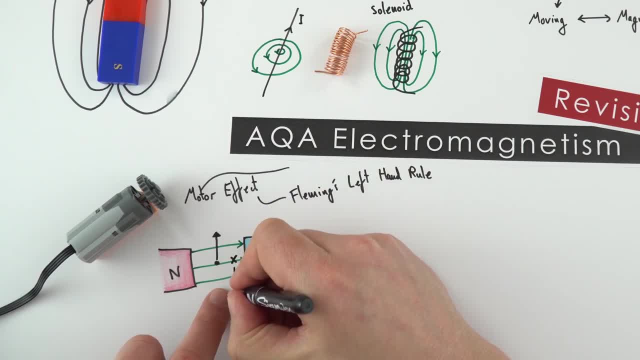 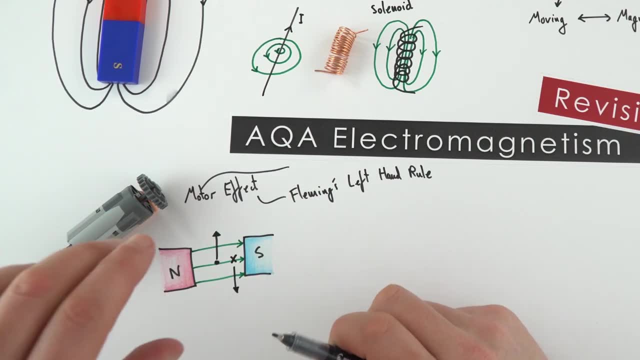 towards you, some of that current is flowing the other way, and what you then have is, as soon as you pass a current, basically the piece of wire, some of it moves up, some of it moves down, and then you can use a thing called a split ring. 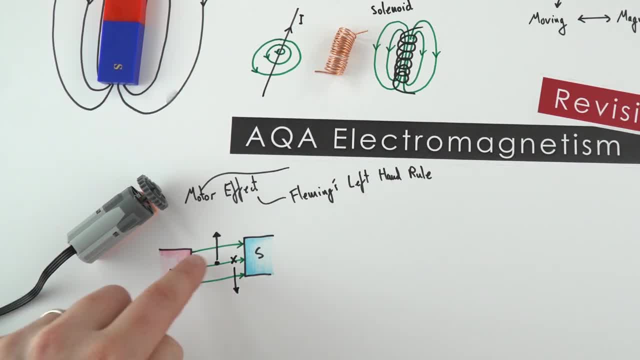 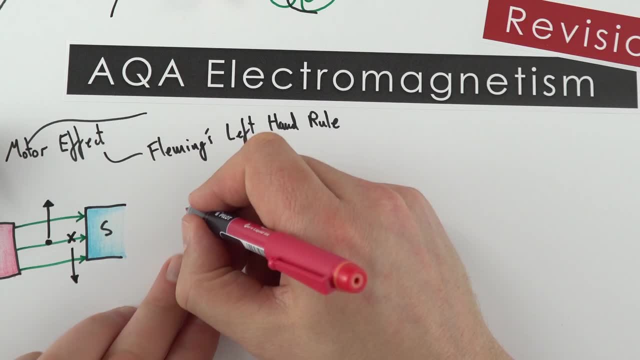 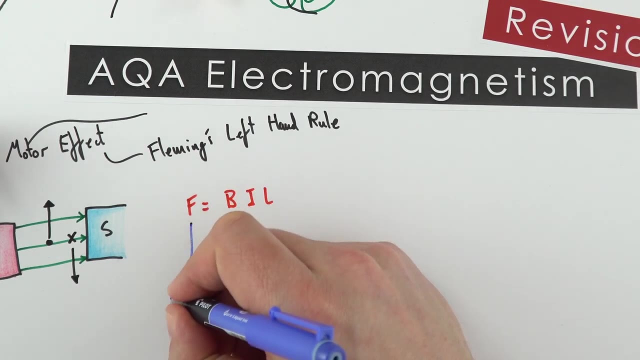 and that allows you to then have electric current flowing always in the same direction inside that motor. We can also use an equation to do some calculations and we can actually look at the size of the force on that conductor, and F is equal to B I L, where we measure our force in Newtons. we measure our 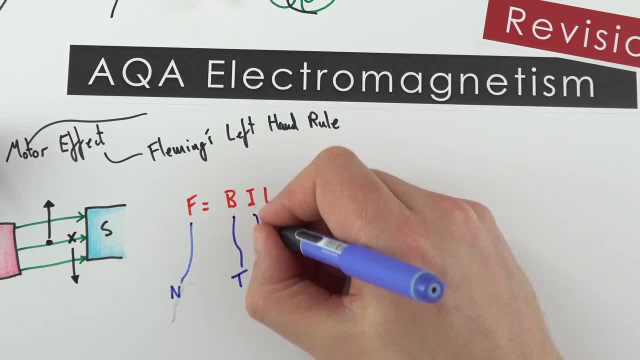 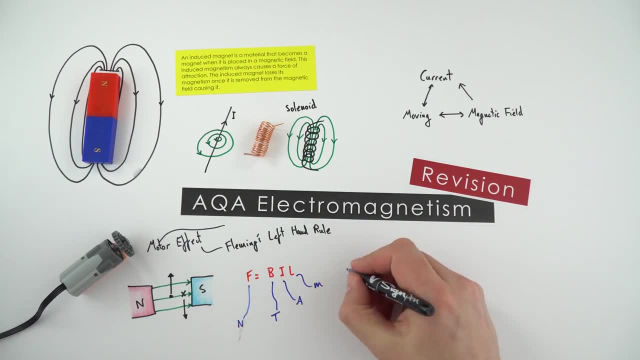 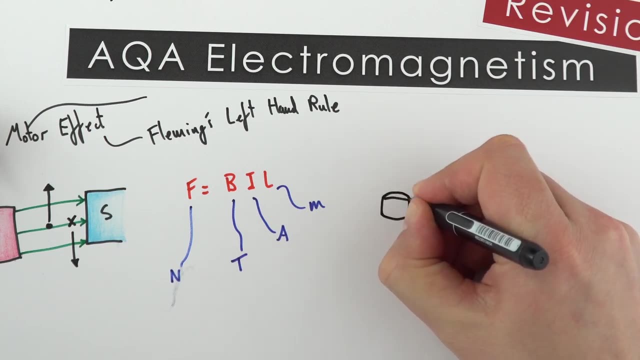 magnetic field and we measure our magnetic field. and we measure our magnetic field in the Tesla, like the car current in amps and length in meters. Now, it's not just motors that use the motor effect. we can also use it in loud speakers. Now, in a loudspeaker you might have a very small circular magnet like 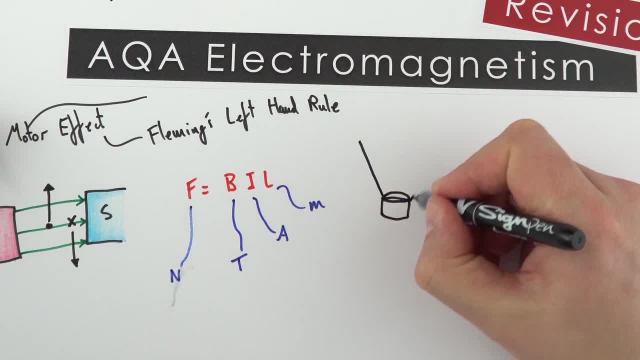 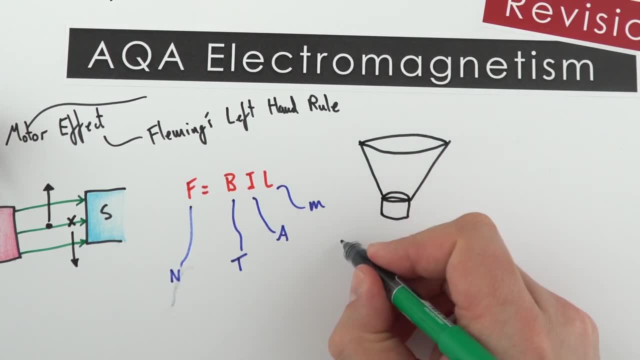 this, okay, and this is connected to, maybe, a large paper or cardboard cone. Okay, so you've got your magnet at the bottom. What you then do is you have a coil of wire that comes in and it's connected to a magnet and it's connected to a magnet. 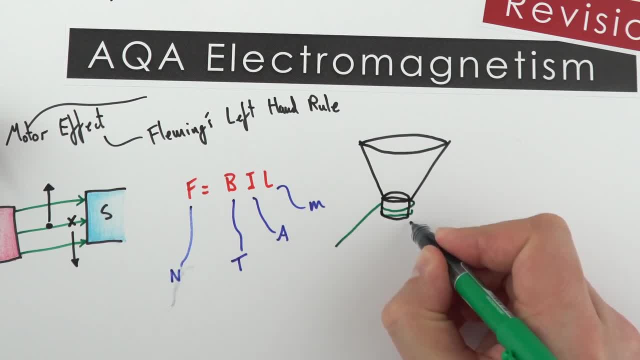 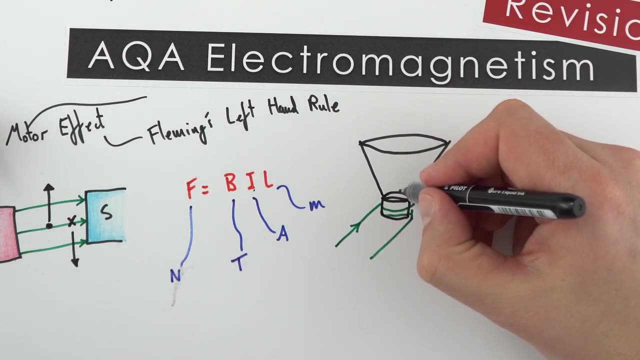 It comes in and it goes around this several times. Okay, now what happens is that if you have a current flowing in one direction, you've got a current flowing, you've got a magnetic field in this permanent magnet down here, and what that means is that maybe, when the current flows this way, the thing here 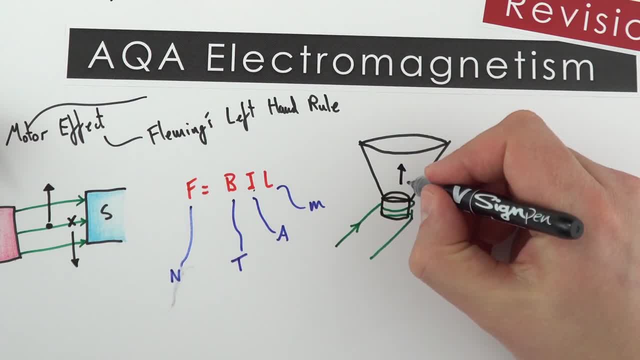 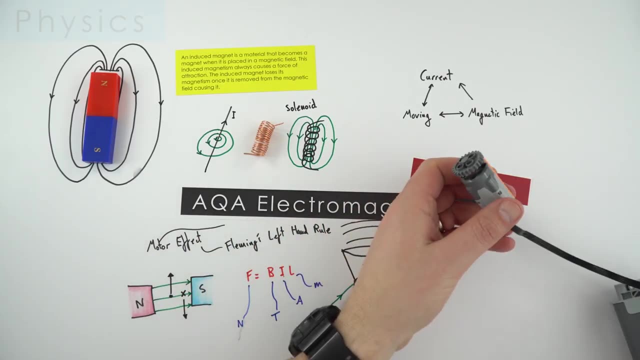 moves up. If you then have the current flowing in the other direction, it moves down, And by varying very quickly which way the current is flowing, that causes the speaker to move up and down, which then causes a load of sound waves to be radiated from this. but this doesn't have to just 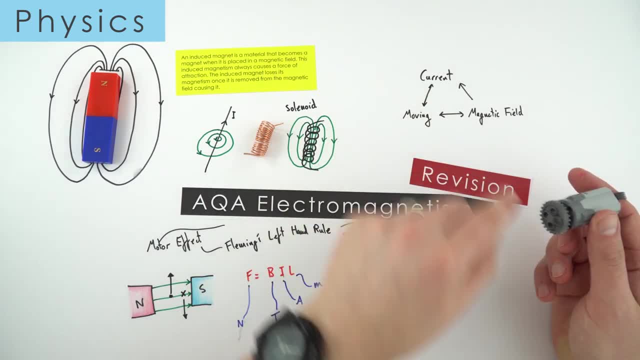 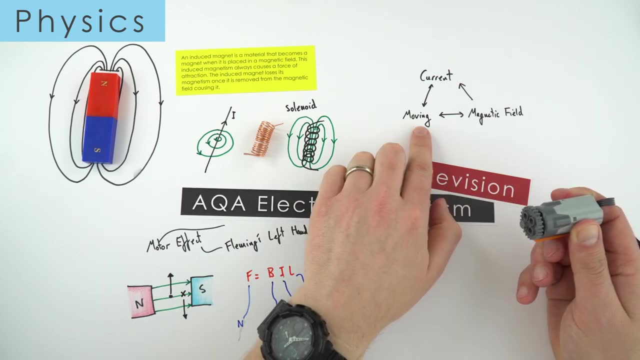 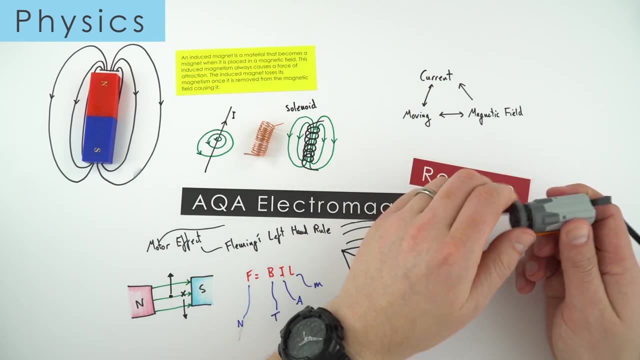 be a motor if we think about maybe moving this thing inside a magnetic field. what we're now doing is we are using this as a generator. so by moving this conductor inside a magnetic field, we induce a potential difference and therefore we induce a current. so a motor and a generator. 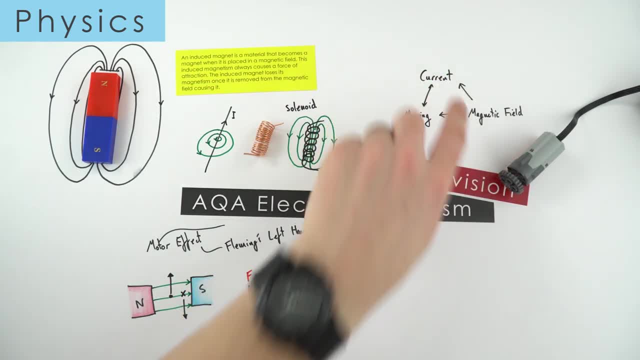 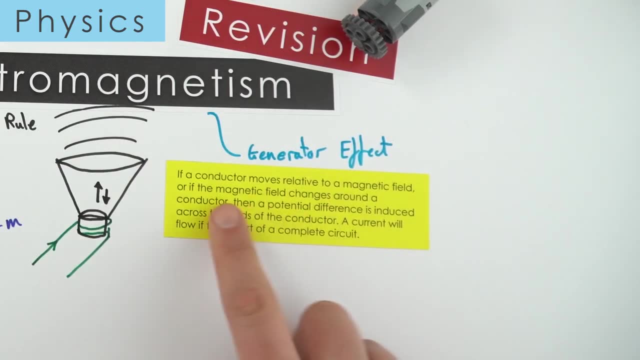 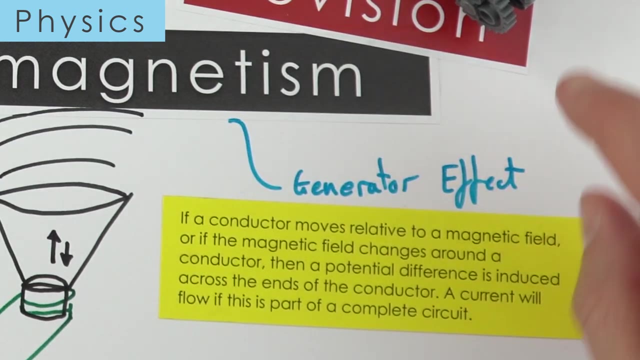 are very, very similar. again, all we're doing now is completing, i guess, the other side of that triangle, so we can also think about the generator effect. so with the generator effect, if a conductor moves relative to a magnetic field or the magnetic field around a conductor changes, then we induce a. 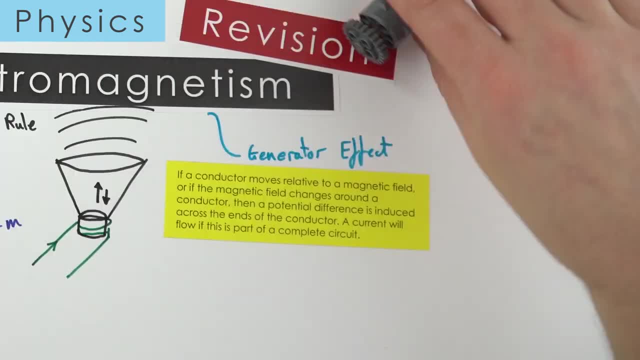 potential difference across the ends of the conductor, and this is if this is then part of a complete circuit. we then have a current that flows. so how do you make this effect bigger? how do we get more electricity out of our generators? well, one thing we can do is we can increase the size of the magnetic field, so you make the 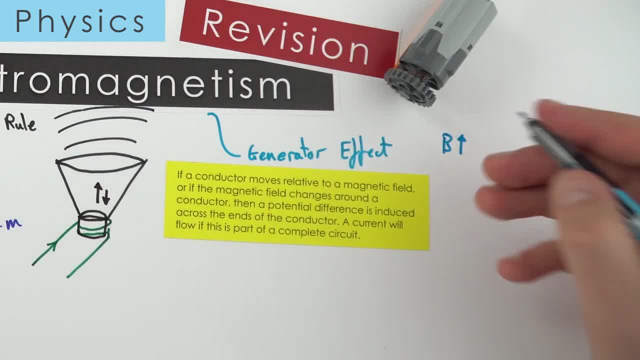 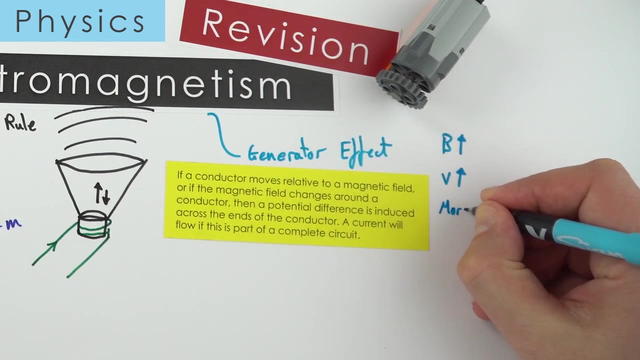 magnetic field bigger, it's going to cause a bigger voltage. you can also make it move quicker. so v is our velocity here, or speed. so we can move something quicker. and also we can have, if you had maybe a coil of wire which is turning inside the magnetic field. what you can do is you can have more turns. 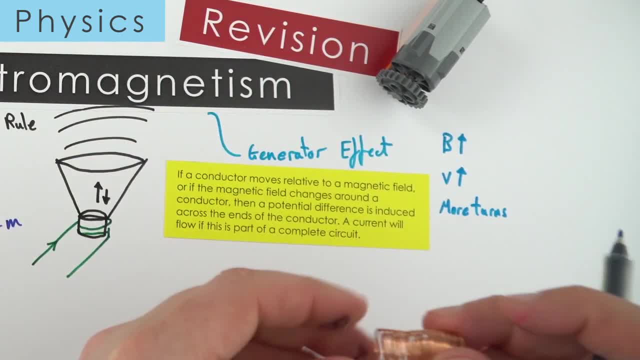 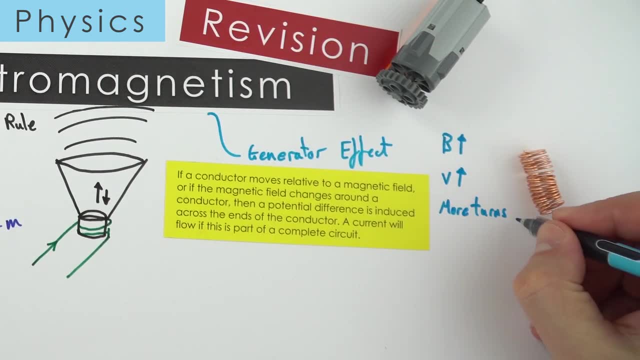 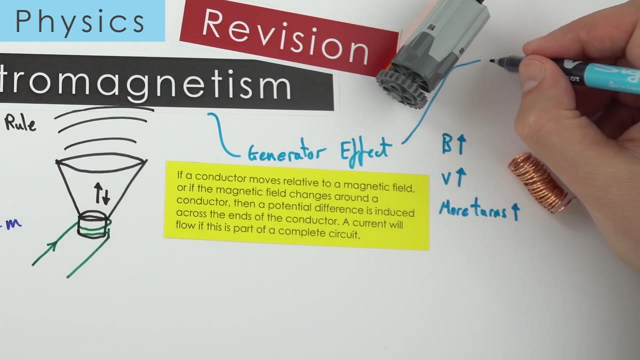 so this solenoid here has one coil of wire, but the amount of time that it goes around gives us a number of turns. so if you have more turns on the generator, that's going to cause there to be a bigger induced potential difference. now, generators are really two sorts. we have things 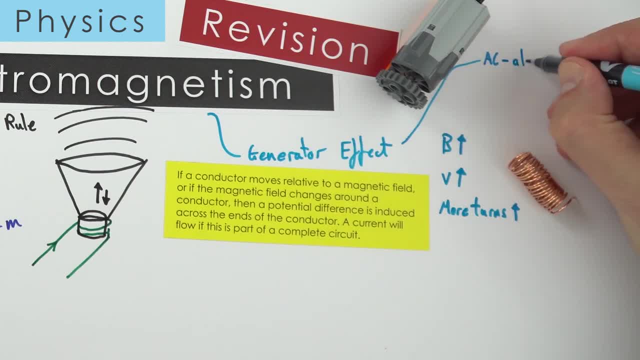 which are ac, so alternating current, and this is called an alternator. but you can also have ones which give a dc supply, and this is called a dynamo. and if we were to look at the output voltage with time, what we'd see is for an alternator. you get something that looks like this: 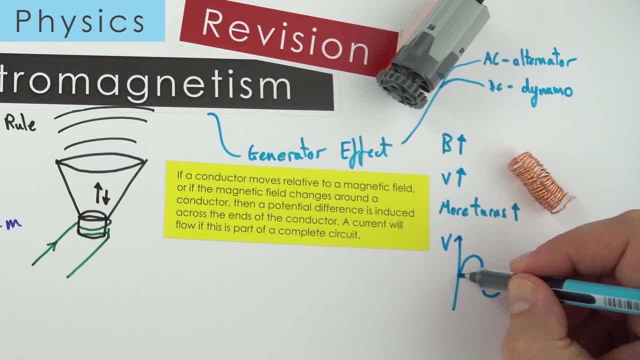 now, if you were to spin it quicker or you had a bigger magnetic field, what we'd then have is a higher voltage, but if it's spinning quicker, then we'd have more cycles per second. and the last thing we're going to look at is the transformer. now a transformer is really useful. 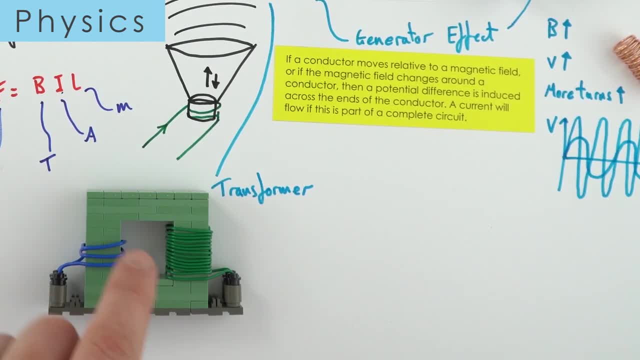 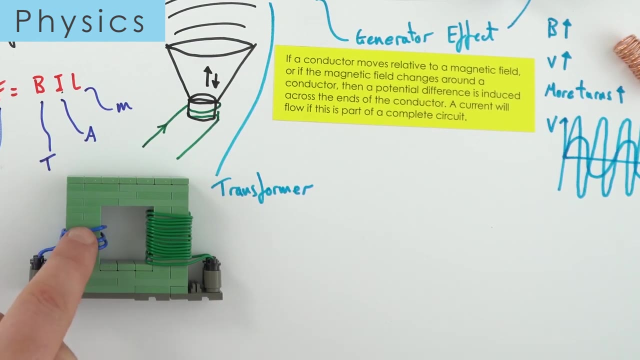 in the national grid, because what it does is it allows us to change the current and potential difference in a different part of a circuit. now, what we have here, this is our normal transformer. we have a primary coil and we have a secondary coil, so if this is where the electricity user may be starting, this is our. 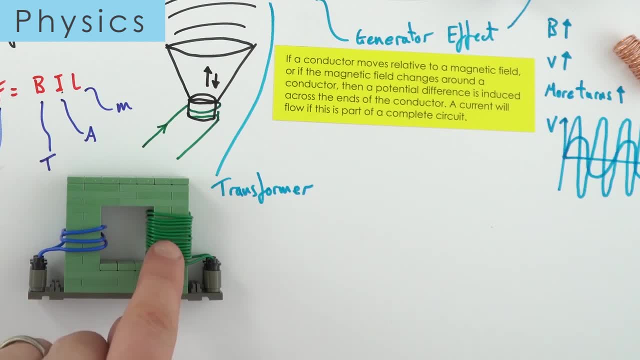 primary coil it's got a number of turns and there's a different number of turns on the secondary coil. so what happens is is that when you have an alternating current in this wire, this causes there to be an alternating magnetic field, like we saw the solenoid up here inside this iron core. 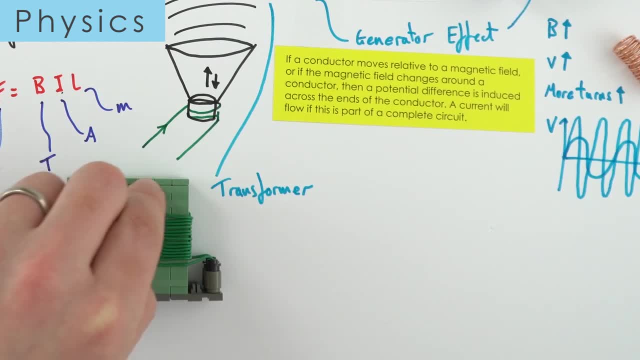 so this iron core then becomes magnetized and what we have is the current, is the magnetic field moves this way and then moves that way, and that's what we're going to look at here and we're going to look at weight. What we then have is this iron core transmits that magnetic field to the secondary. 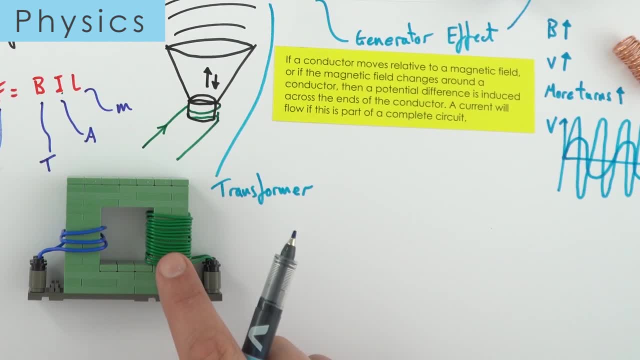 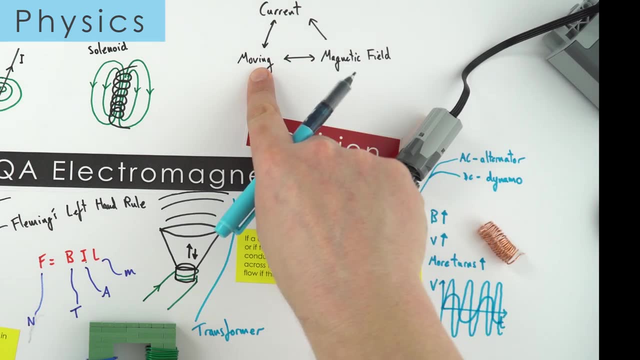 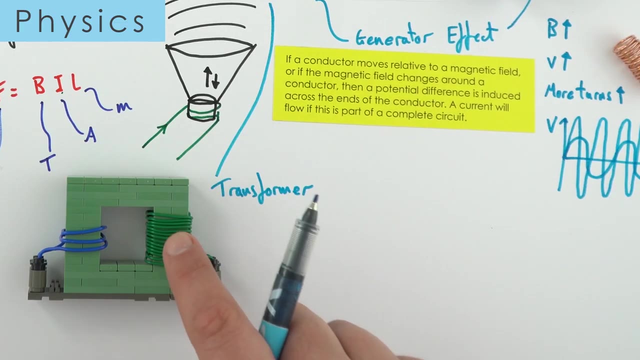 core. So inside this coil of wire we then have a changing magnetic field. If you've got a changing magnetic field, which is effectively that magnetic field is moving, we then induce a potential difference. So we then have a potential difference in the secondary coil which causes a current to. 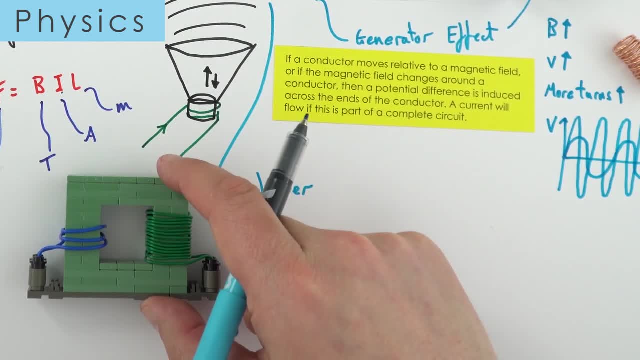 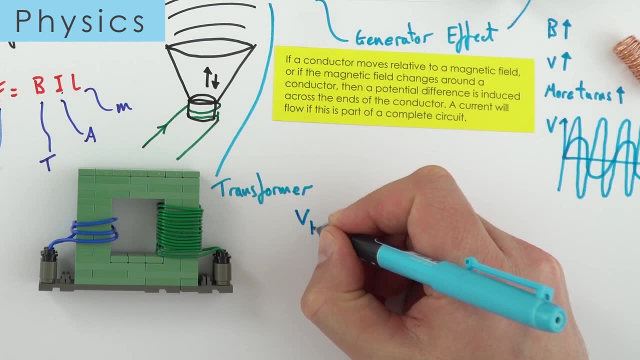 float. So that is the kind of bog standard average transformer that you need to know about for GCSE. So with this we can think about the potential difference in the primary coil, we can think about the current in the primary coil and also the number of turns on the primary coil and obviously 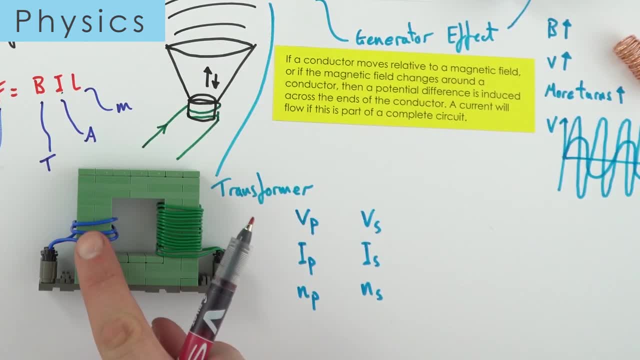 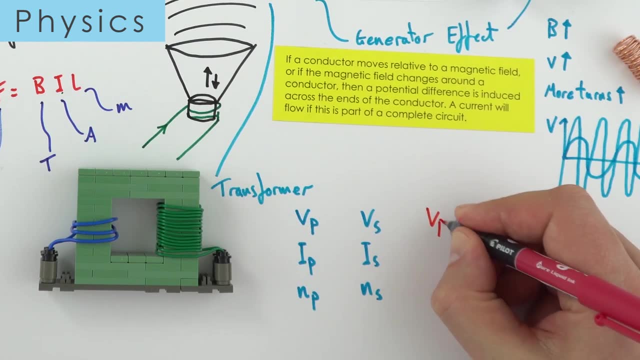 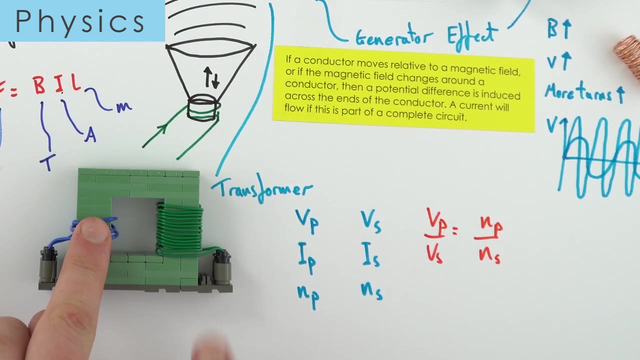 we can do the same for the secondary, And what we find is that the potential difference increases in proportion to the number of turns from the primary to the secondary. So what we can say is that VP over VS is equal to NP over NS. So imagine that had five turns and 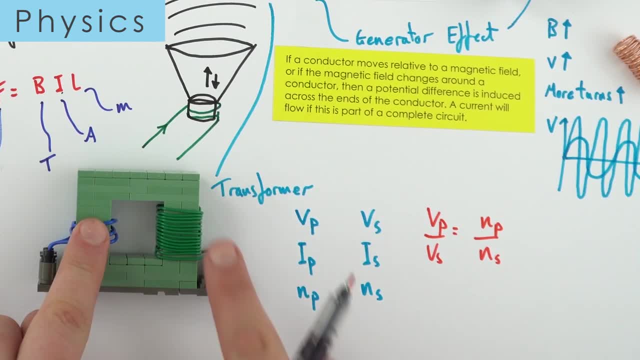 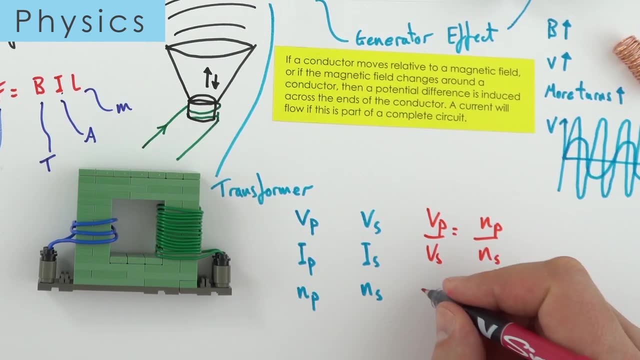 that had ten turns. that means you might go from 5 volts to 10 volts, But when you increase that potential difference, we reduce the current, And the other equation we can say is that VPIP is equal to VSIS. So this is effectively power, remembering that power is equal to potential difference times. 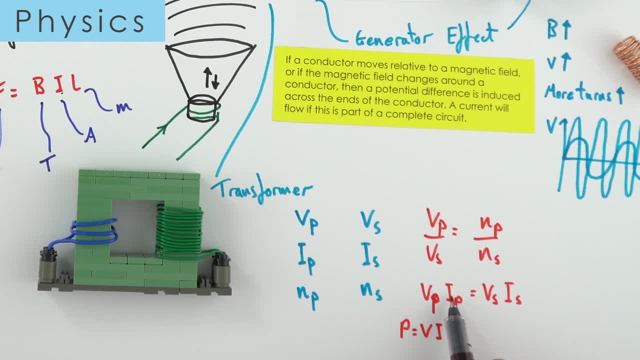 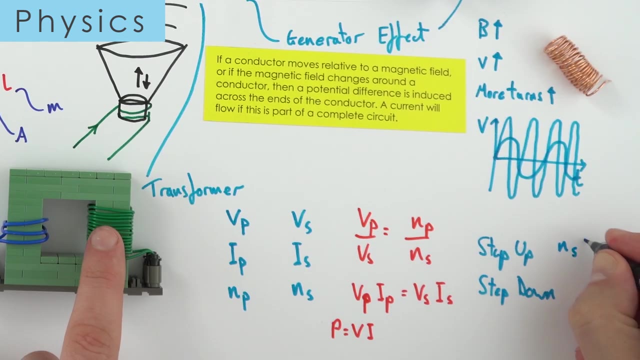 current. If you've got a power coming in, it's the same as the power going out, and that means that the initial power on the primary coil is the same as the power on the secondary coil. Now, on a step up transformer, it steps up the potential difference, so that means there's a bigger number of turns on.